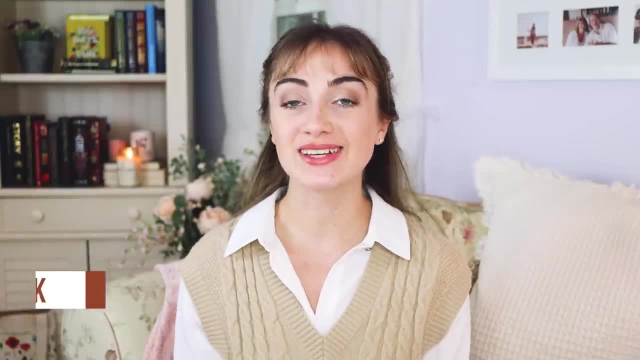 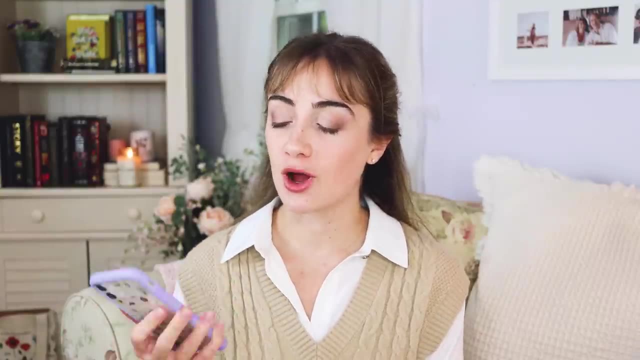 What's up my friend Abbey here and welcome back to Ask Abbey, where I answer your writing questions and help you make your story matter. Today's question comes from Joshua. First off, thanks for all the work you do to bring this information and advice to us. 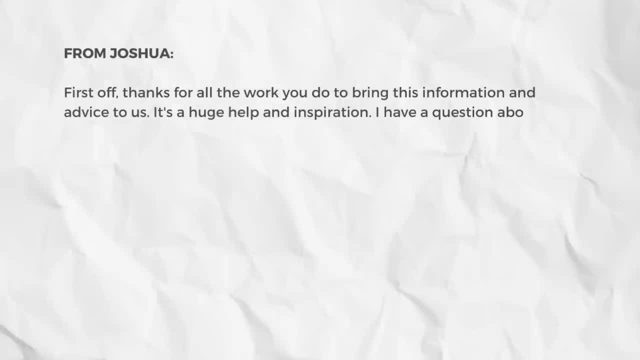 It's a huge help and inspiration. I have a question about creating characters in a series. I understand the concepts of desire, fear and misbelief, but I'm not exactly sure how to balance or prioritize them throughout the series. I guess my question is: how do you know which? 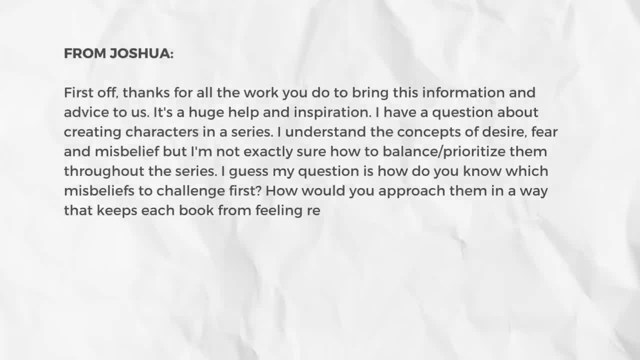 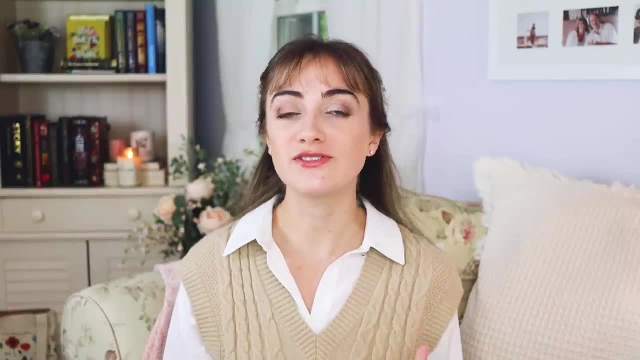 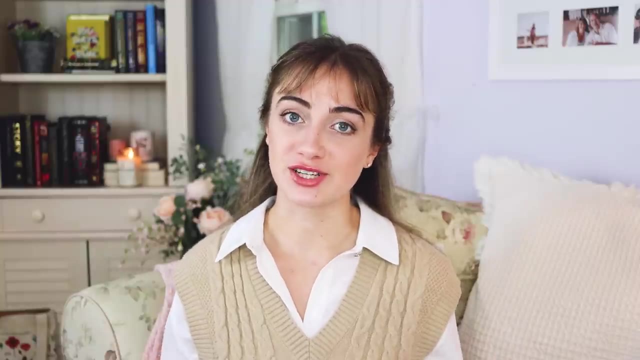 misbeliefs to challenge first? How would you approach them in a way that keeps each book from feeling repetitive? I hope that makes sense. Thanks in advance. That is a great question. It's definitely easier said than done to keep your characters learning and growing and facing new conflicts throughout a series. 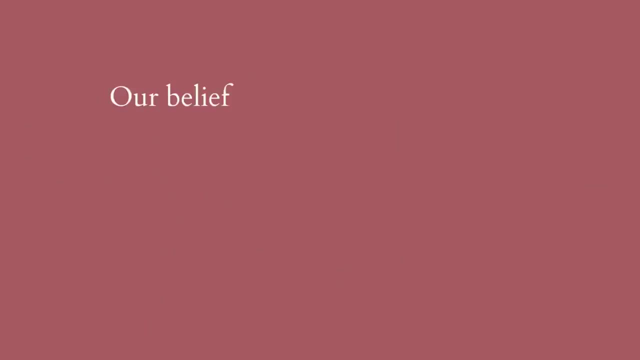 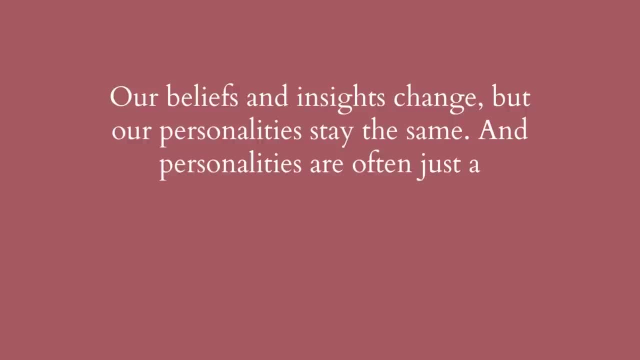 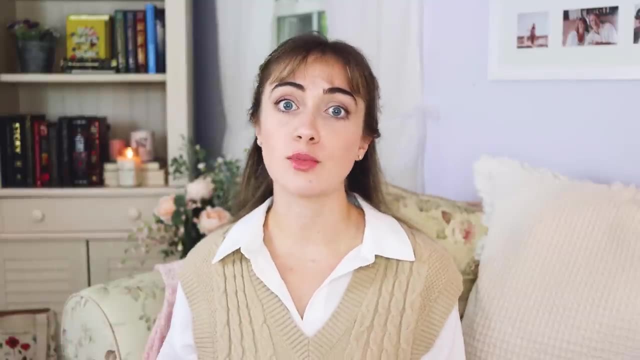 change, but our personalities stay the same, And personalities are often just a combination of strengths and weaknesses. So even if your character goes on a journey and book one has an aha moment and crushes their misbelief, they still have challenges to face because they still 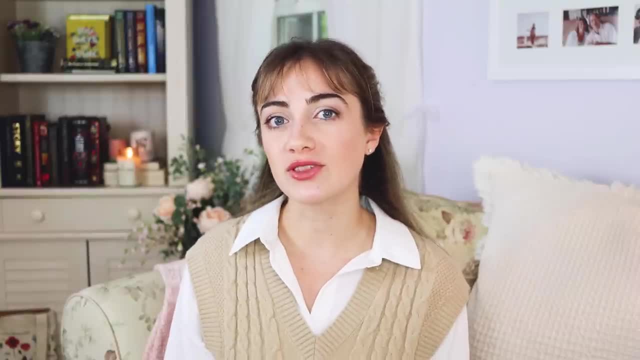 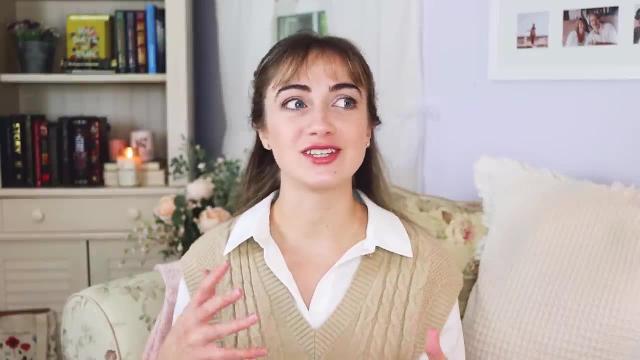 have strengths and weaknesses. That means with each new book they will face new challenges because of who they are as a character, And this is the fun part to me, because this is where you get to play with different types of character arcs. So maybe in book one your MC follows a character. 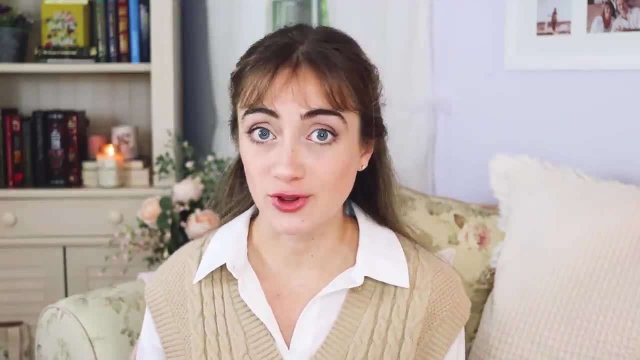 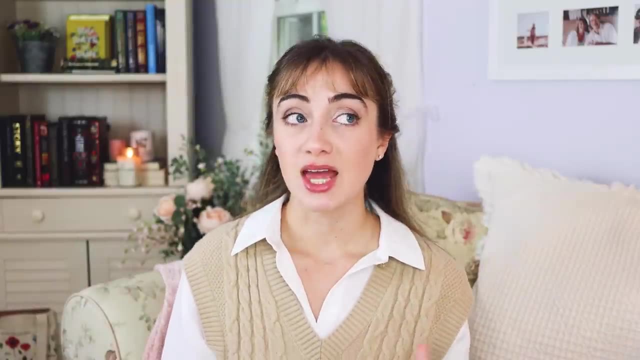 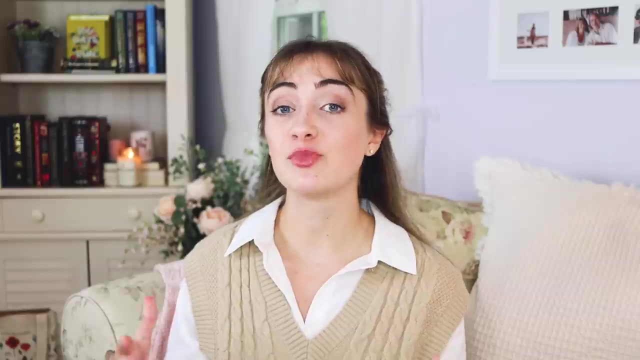 arc of self-discovery and she overcomes a fatal flaw. But then book two forces her to confront a deep-seated fear that she hasn't conquered yet, And maybe she doesn't change for the better at the end of book two, Maybe she dives headlong into a disaster, and then book three is the arc of her. 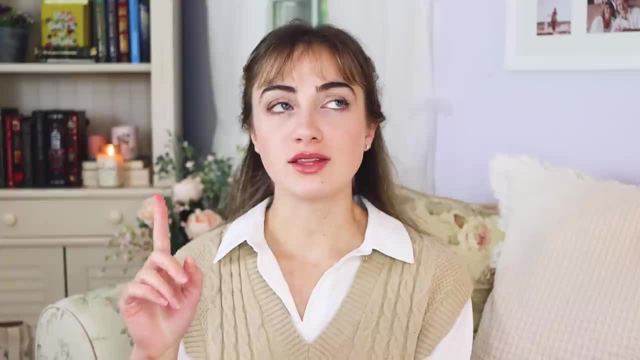 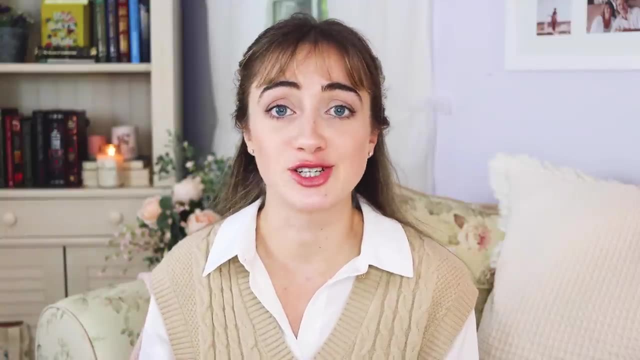 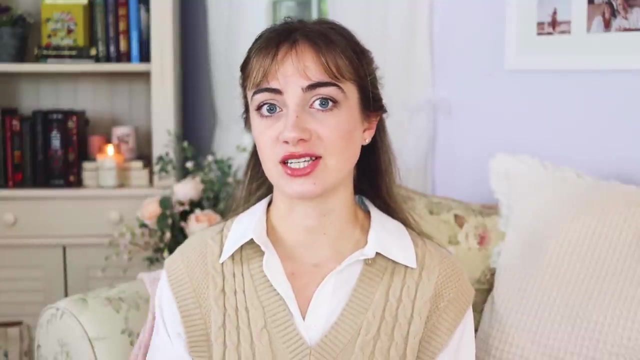 overcoming challenges, to redeem herself. The key to making each book feel not repetitive is pretty simple. It's basically something you have to change. Bring the characters on a journey and leave them in a new place emotionally. That's it. Seriously, Don't overcomplicate it. So I'm in the midst of co-writing a series with 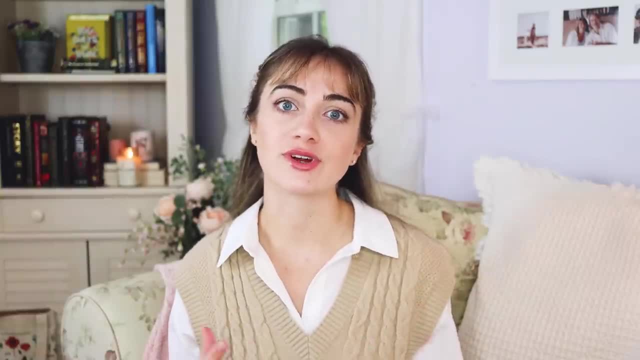 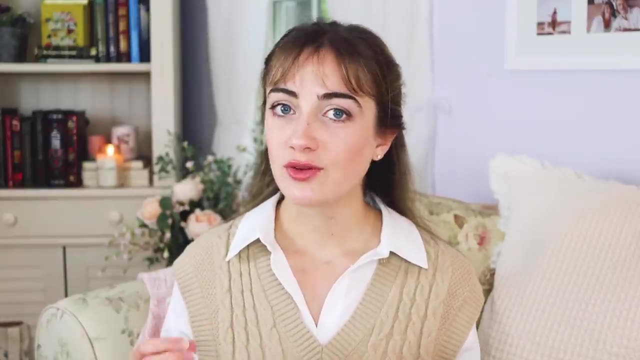 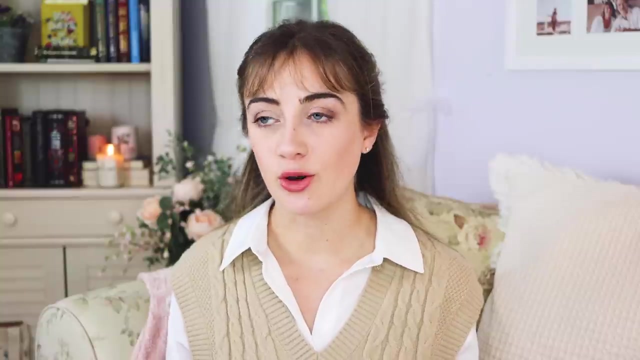 my sister Kate, And as I am outlining and gathering ideas for future books, I keep returning to this concept of strengths and weaknesses, Because, even though the characters are learning and growing and overcoming fears, they always have those strengths and weaknesses. They always have those things that they're really good at and then those things that they're 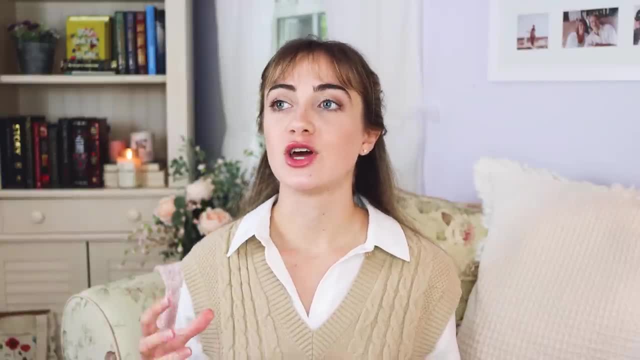 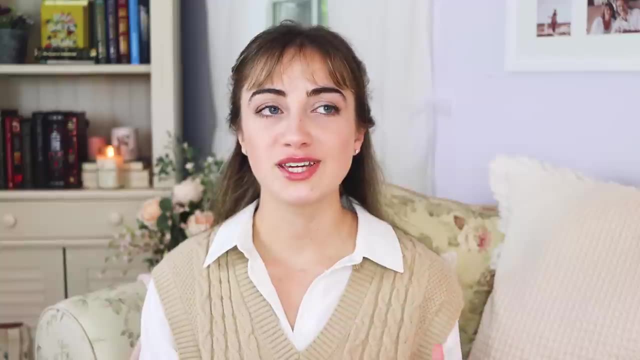 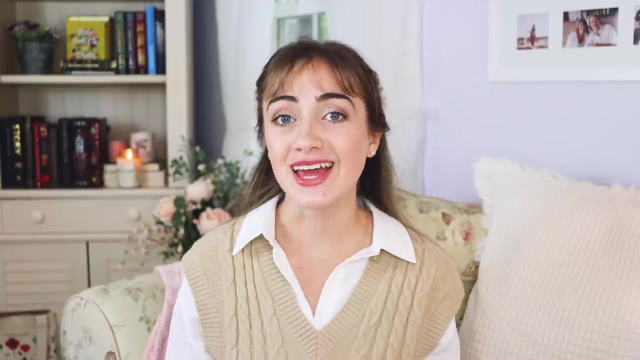 susceptible to. Once you develop their personality and you establish those strong points and those weak points, the story kind of writes itself, Because you have these super flawed, super conflicted characters who have so much to learn And each book can take them on that learning. 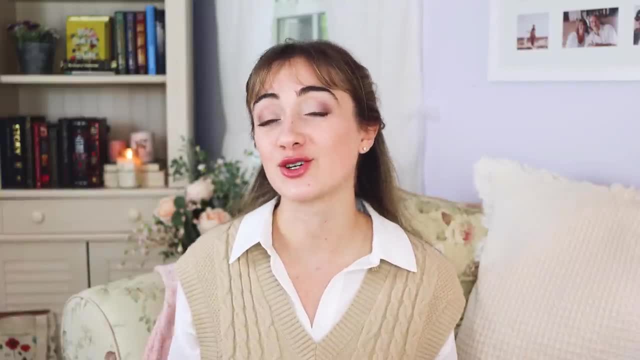 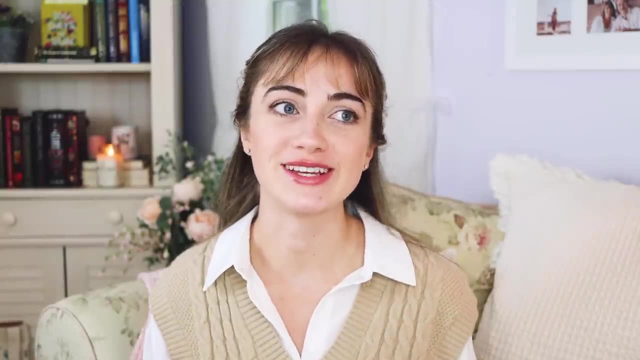 journey in a different way. That's part of what makes a cast of characters interesting to watch as they interact with each other. So I'm in the midst of co-writing a series with my sister. each other When each character is known for something, whether it is their fears, their vices. 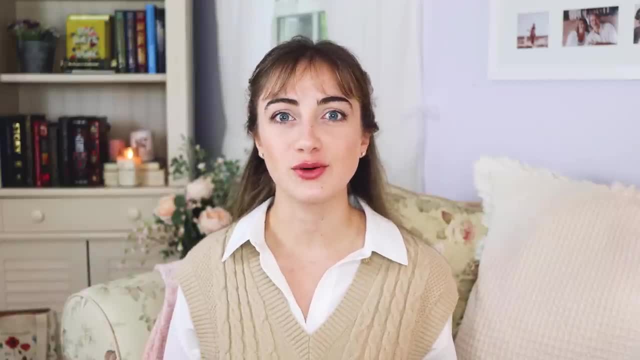 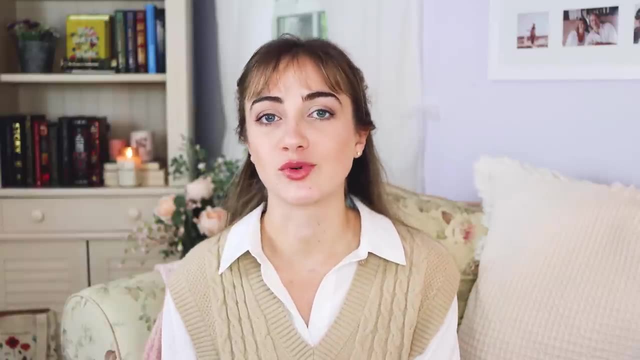 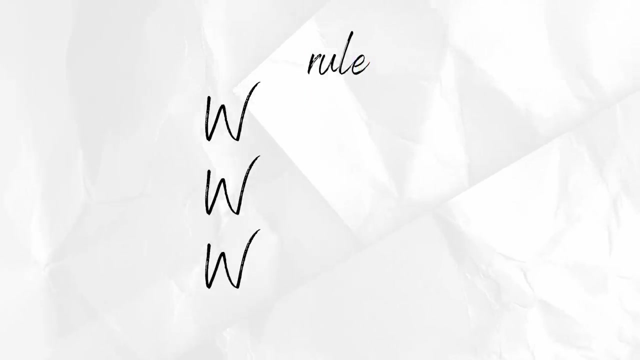 their virtues. it creates that opportunity for humor and relationship building between the characters, rather than just everyone being a little boring cardboard cutout with the same exact stakes. I like to call this the WWW rule, giving each character a weapon, a weakness and a want. 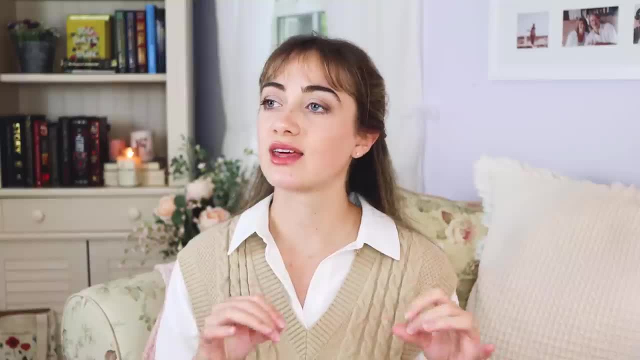 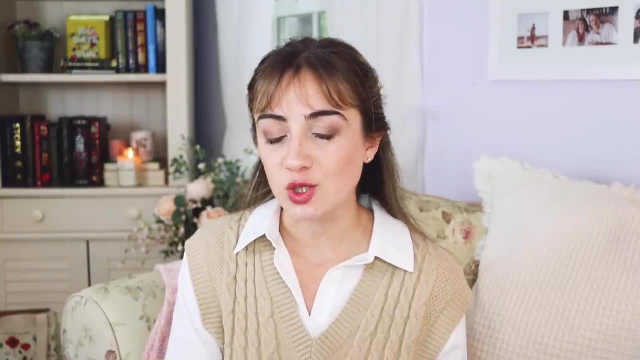 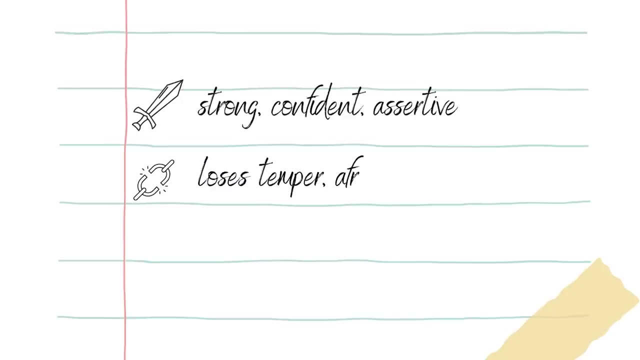 These are fundamental elements of your character, meaning they never change that much. They are what defines your character. For example, let's say you have a character whose weapon is that they are strong, self-confident and assertive. Maybe their weakness is that they 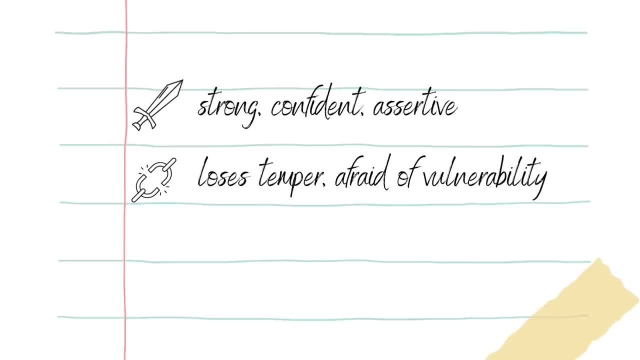 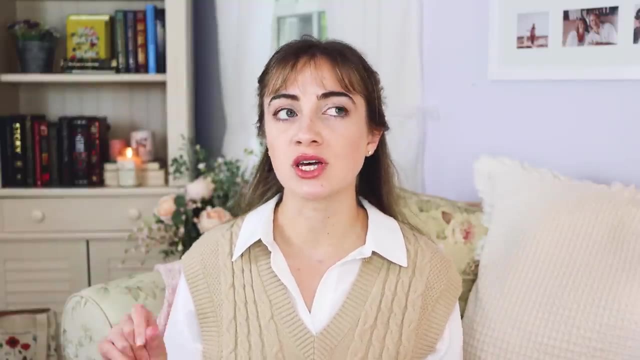 lose their temper easily and have a hard time being vulnerable with others. Their fundamental want is to feel safe and protected, both physically and emotionally. These are fundamentals at your character's core, which means even if they go on a transformative journey and change as a result, they will still have these core characteristics. 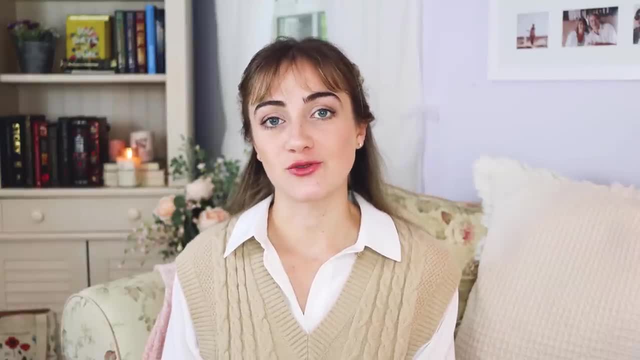 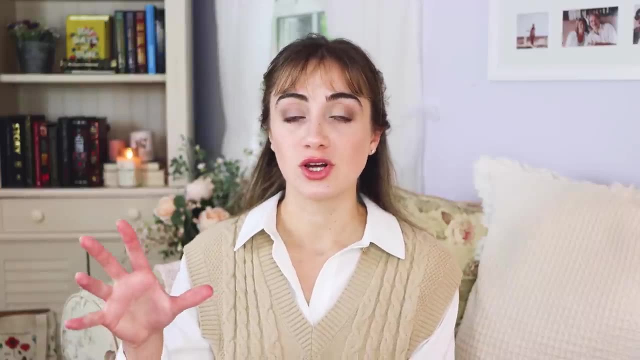 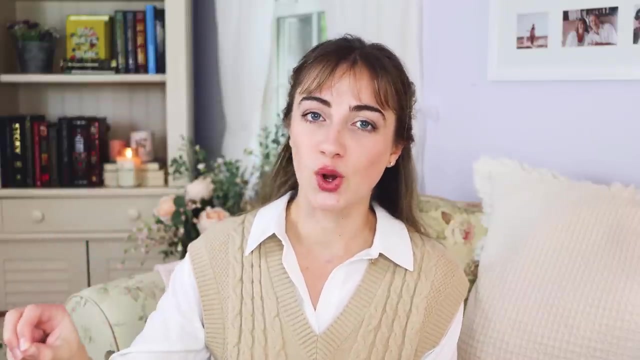 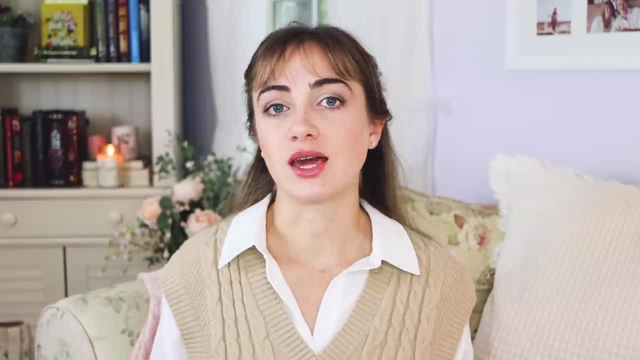 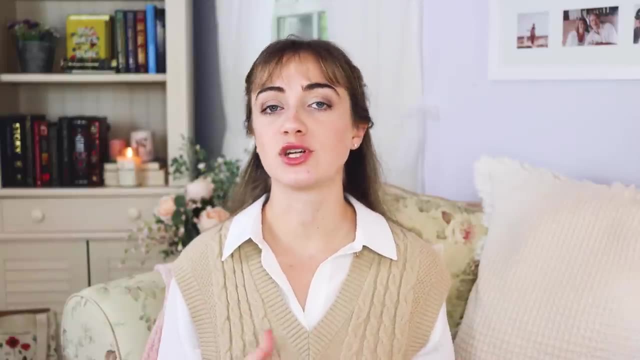 new things, But we're always fundamentally kind of the same. We always return to pretty much the same personality. Now, there are different levels to each Enneagram Type, ranging from healthy to unhealthy, which can also be really helpful when developing longer character arcs. 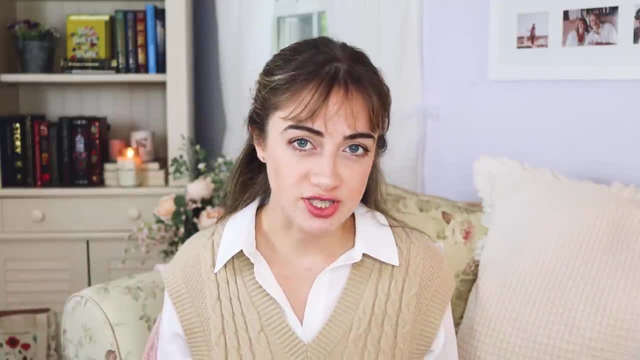 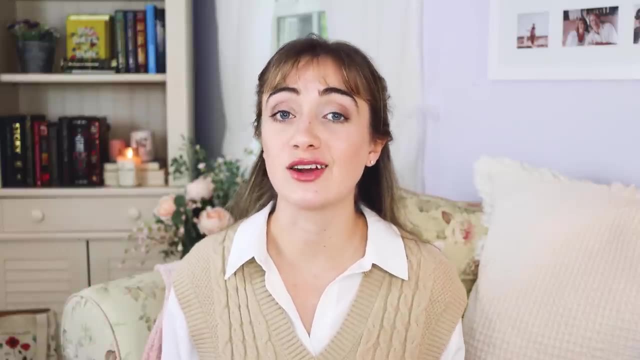 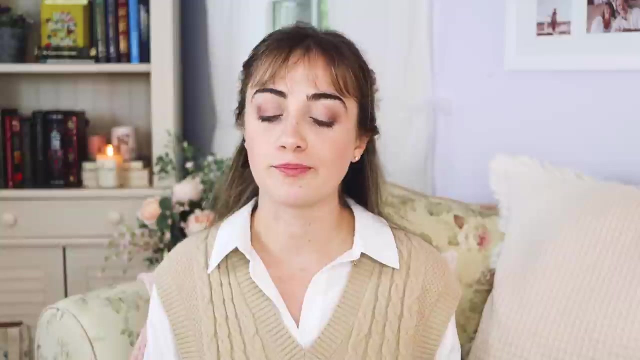 especially character arcs that kind of stretch over the course of an entire series, And these transformations may be for better or maybe for worse. For example, let's look at the differences between the healthy Enneagram 8, the average Enneagram 8, and the unhealthy Enneagram 8.. This is taken from psychologyjunkiecom. 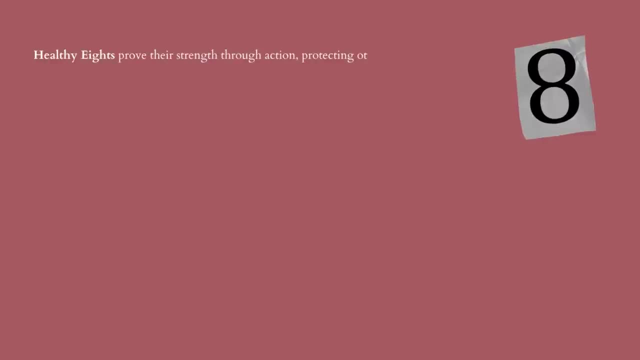 Healthy 8s prove their strength through action, protecting others and bringing out others' strengths. They let go of the belief that they always have to be in control of their environment, which lets them look inwards, to their hearts. They are strategic, decisive and resourceful. 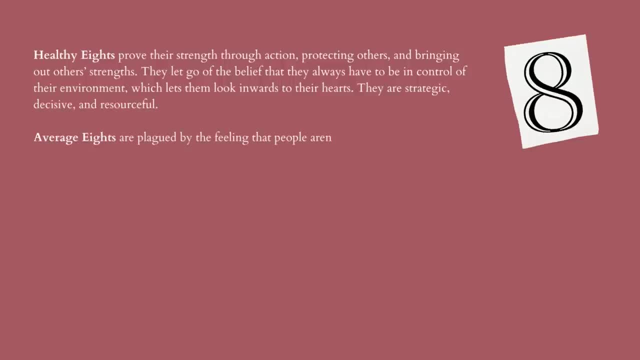 Average 8s- are plagued by the feeling that people aren't loyal or respectful to them, so they try to convince others of how important they are. They can be both boastful, willful and proud. They are typically shrewd and efficient at getting what they want. 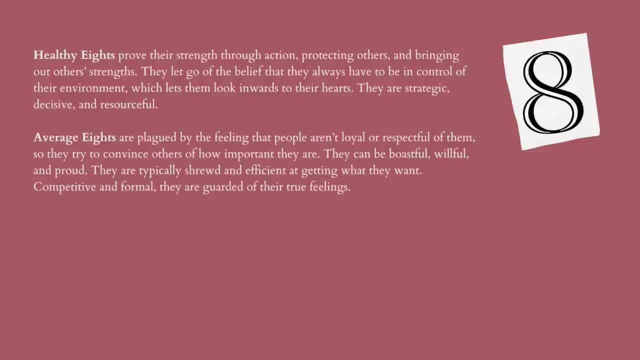 Competitive and formal. they are guarded of their true feelings. Unhealthy 8s feel like people are turning against them, so they feel betrayed and scared to trust anyone. They feel they must protect themselves at all costs. They can become vengeful, confrontational and intimidating. They may go on rampages. 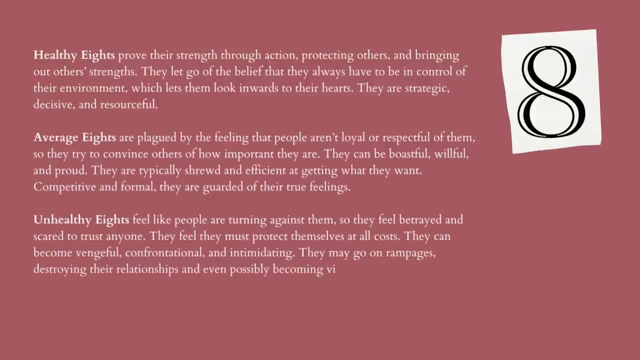 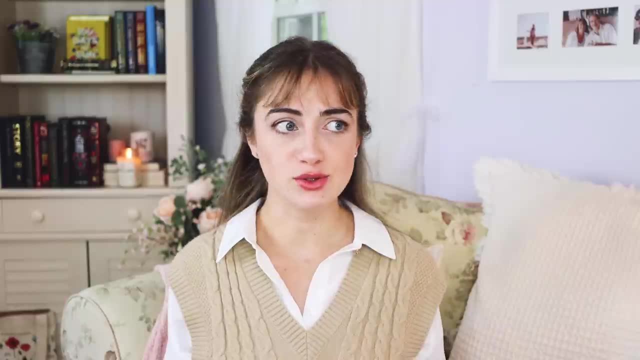 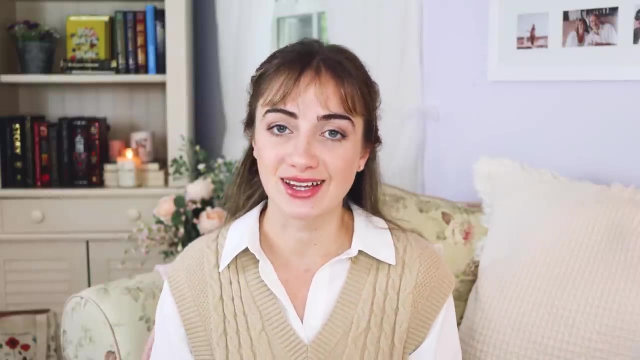 destroying their relationships and even possibly becoming violent. So you can definitely get creative with this. Don't feel like you have to follow the Enneagram descriptions to the letter- Absolutely not. Every person is unique and doesn't exactly perfectly fit into a type, just like every character is unique and doesn't. 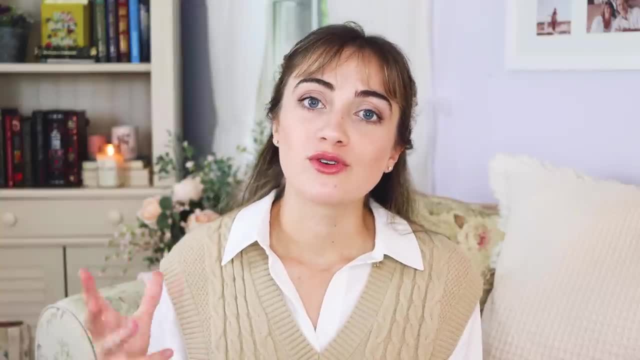 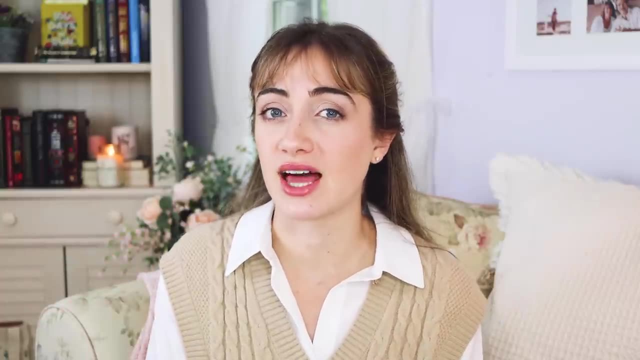 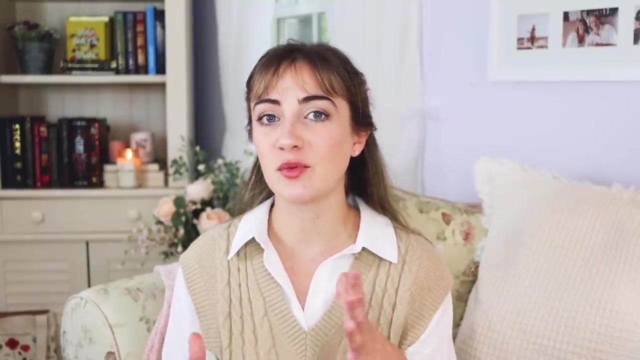 perfectly fit into a type, But it would be worthwhile to write your own descriptions of these healthy, unhealthy, average versions of your character's personality. What would they look like at their best? What would they look like at their worst? What would they look like somewhere in between, kind of struggling between healthy and unhealthy?